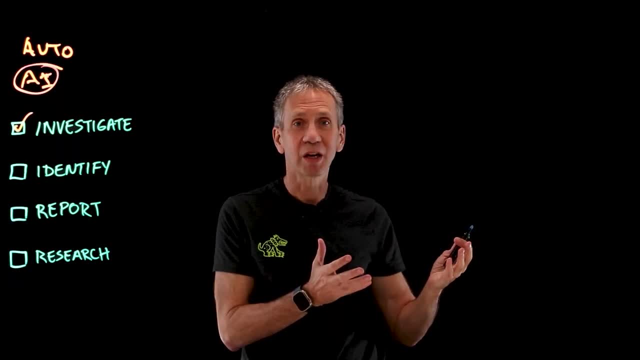 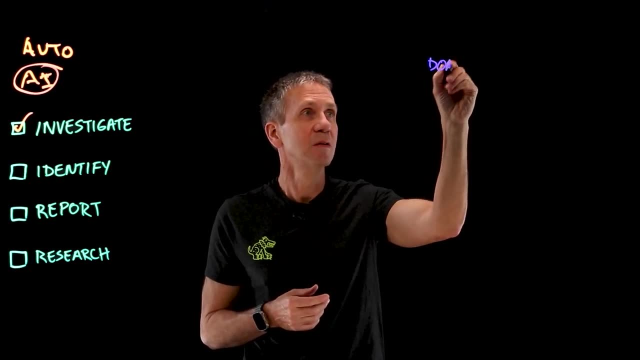 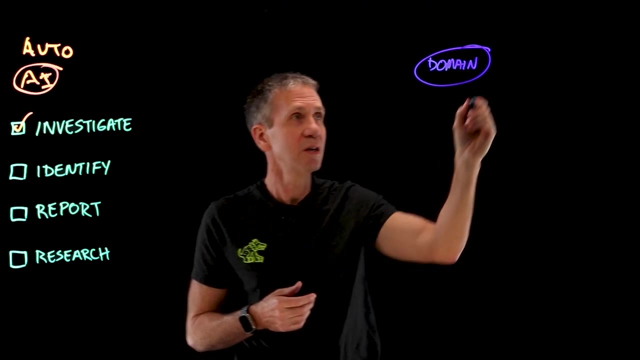 information about the physical or logical world, but representing it as a data structure. And the way this works is to give you an example, Let's say we have a domain and this would be like the name of a web domain, And that domain then resolves to. 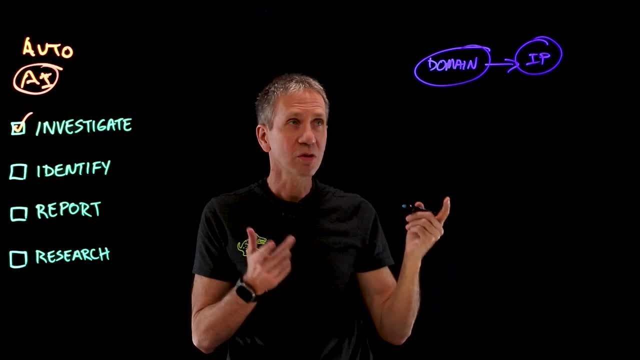 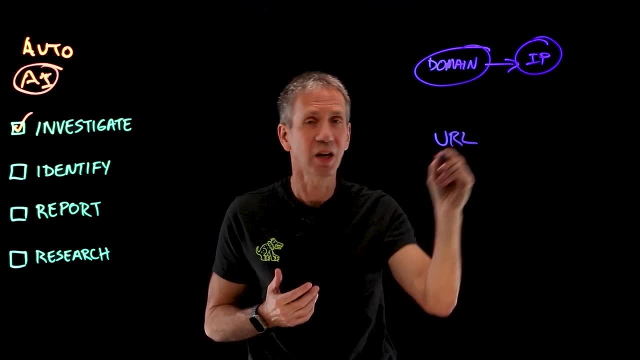 a particular problem, And we can use AI to investigate a particular problem. Now take är and theار IP address Also. so this is what we normally have with the website. Now, what else do we have? Well, we might also have a URL. that's the actual link. 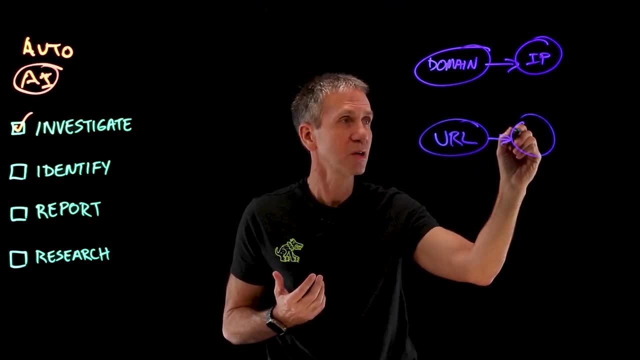 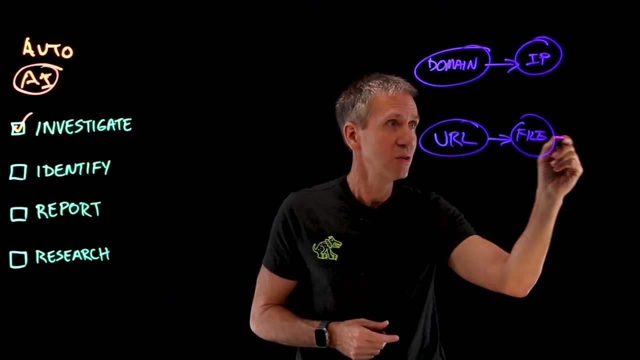 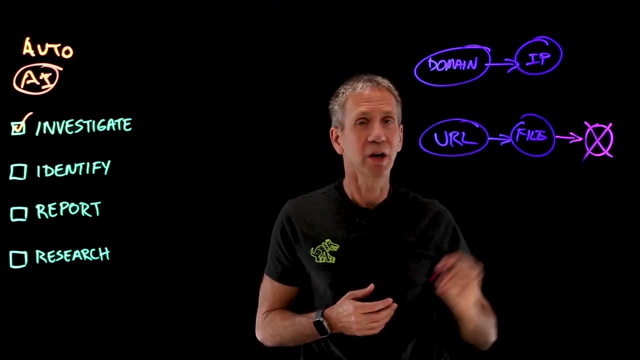 you're going to type into your browser and that is going to link to a particular file on the file system. Now let's take, for instance, if that file on the file system ends up pointing because we know through an AV signature, an antivirus signature, what if this points to malware? 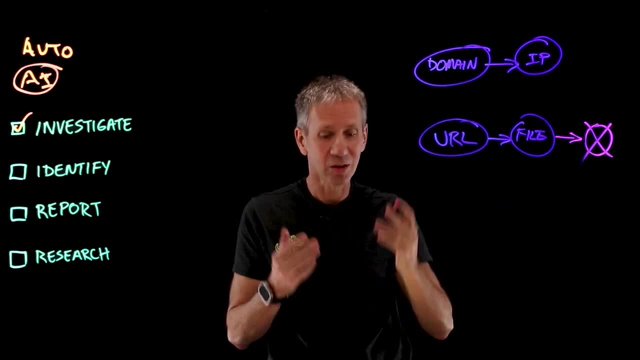 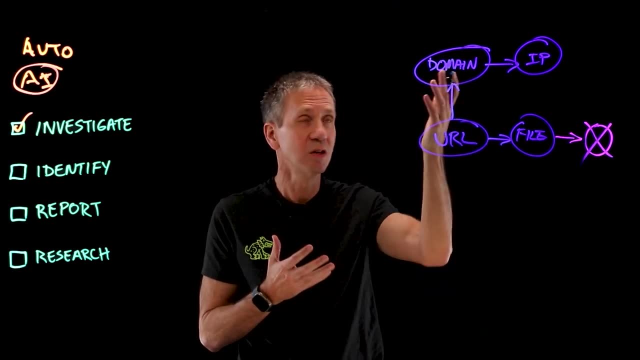 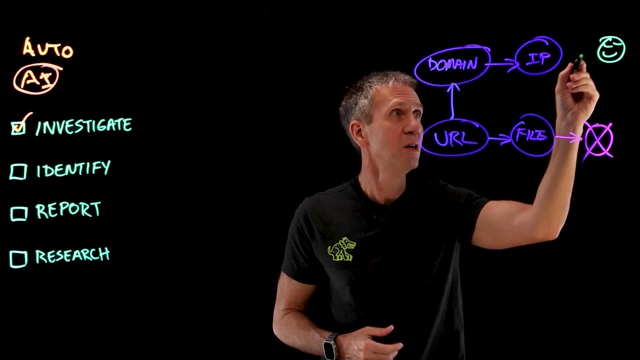 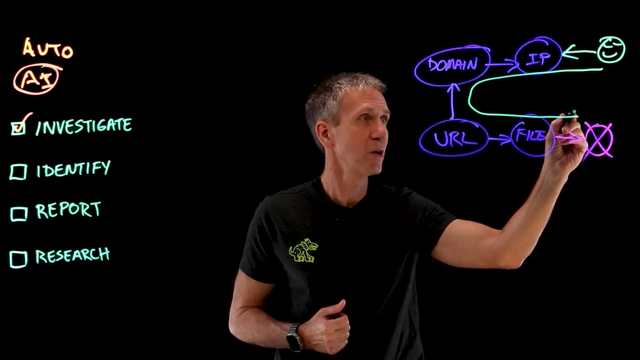 then this is some information that we can now connect together. Then, if we say that this URL is in fact contained by that domain, and then I add a user out here unsuspecting, who connects then to this IP address, then all of a sudden I have a path that goes all the way through from this user to this malware. 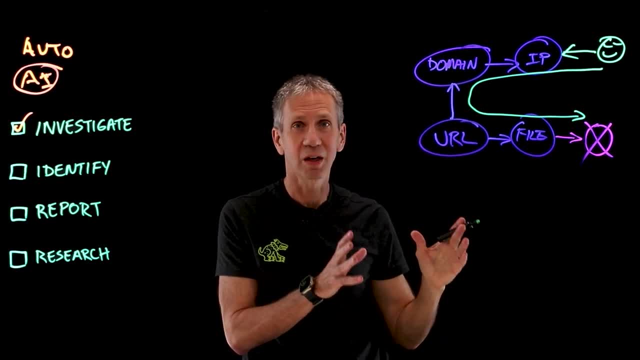 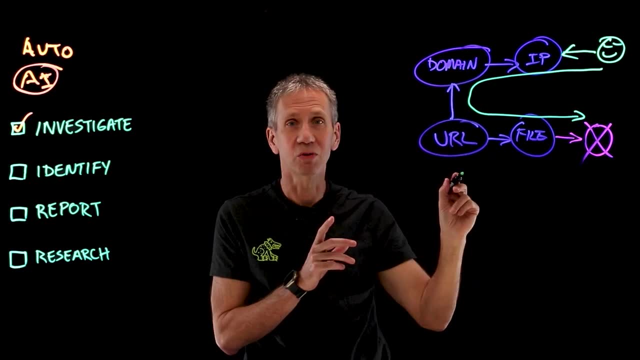 And now I have this data structure that has represented, in fact, the connection that occurred. I now know this user has been infected by this malware and here's the path it took to get there. And, in fact, if this knowledge graph is good enough, 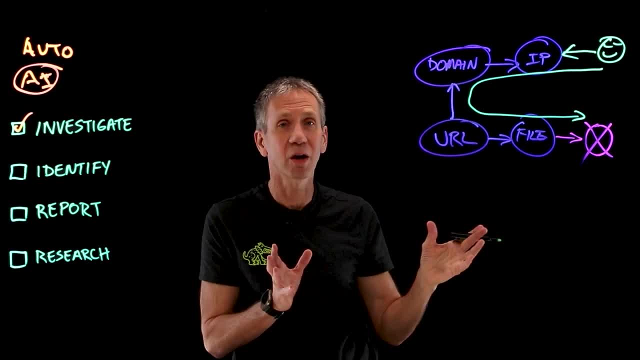 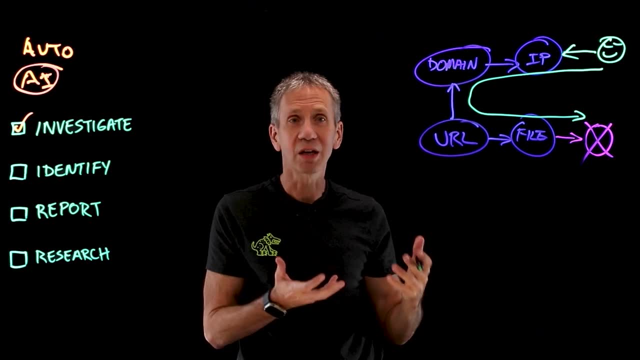 I'll be able to look and see what other users might also be affected, and what other malware and what other sites. So this is a way of representing information and then we can do some reasoning over that in order to do inference. Now, this is how an AIO 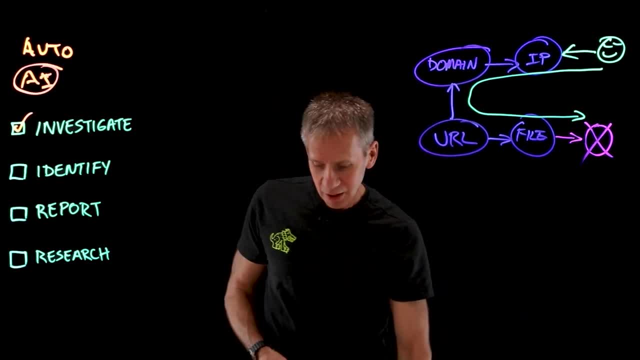 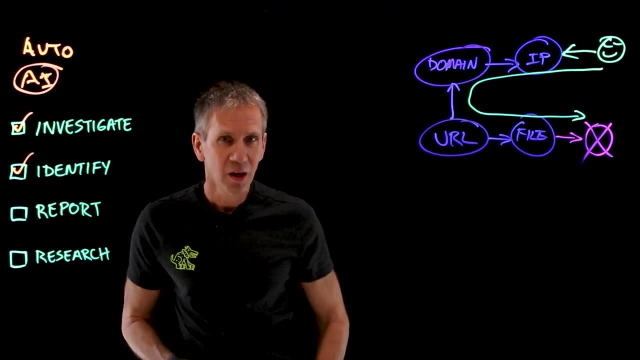 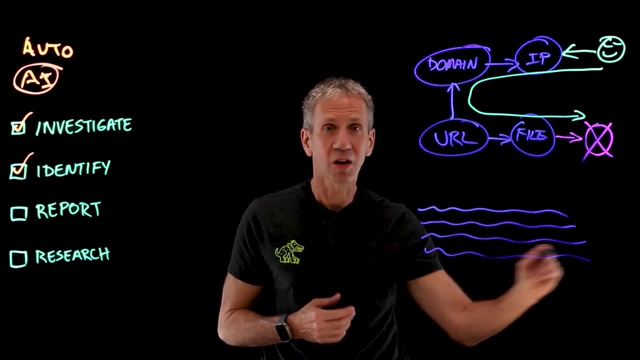 AI system might do this internally. Now that's one way we can do investigation. How about to identify in more detail a particular problem? So systems will typically write out lots of log records. Once an event occurs on a system, then we cut a log record. 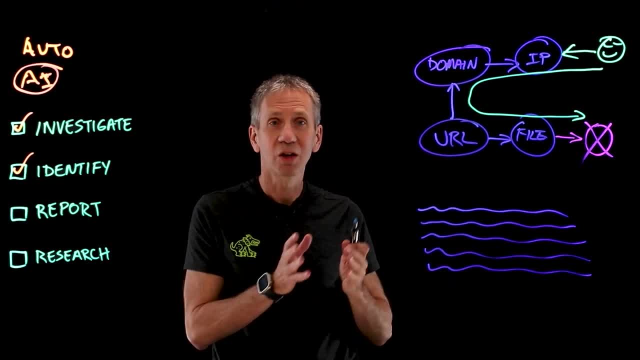 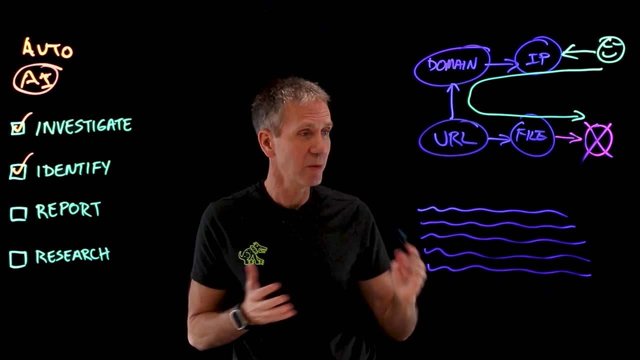 We put out information about: here's the time, the date, here's who did it, here's what they did, here's the system they did it to, here's where they did it from Those kinds of bits of information would be. 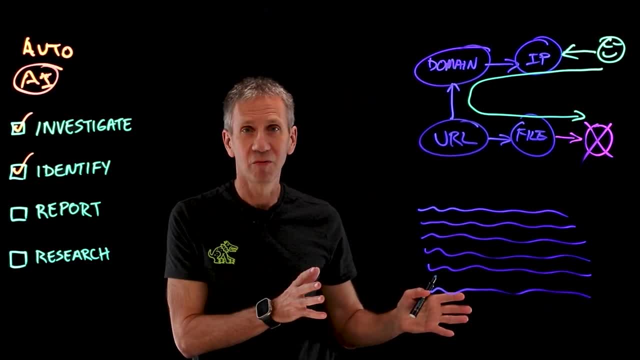 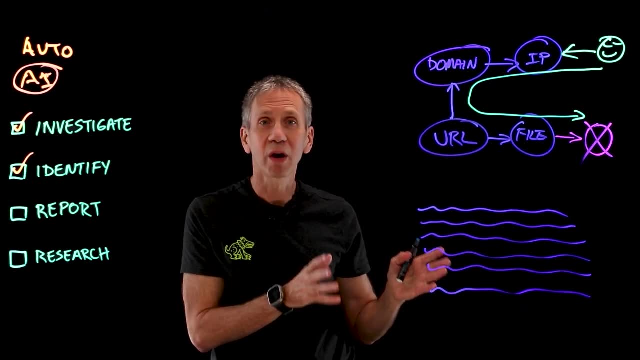 and we would be able to find out what exactly was contained in these log records. And we have loads and loads of these, So it's very difficult to sort through all of that and find where are the anomalous activities, Where are the outliers. 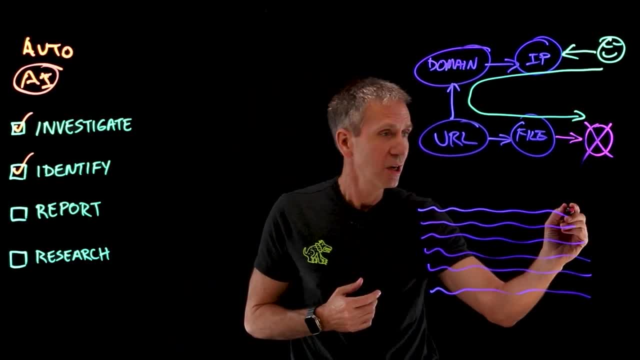 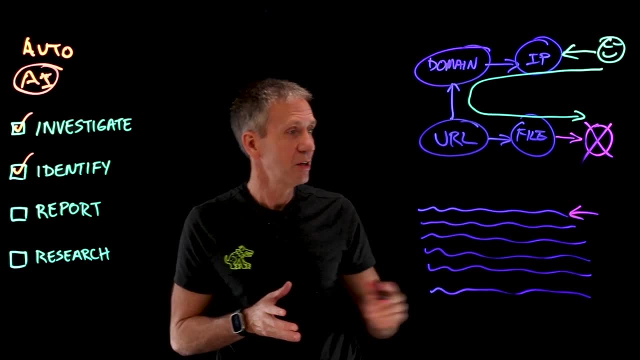 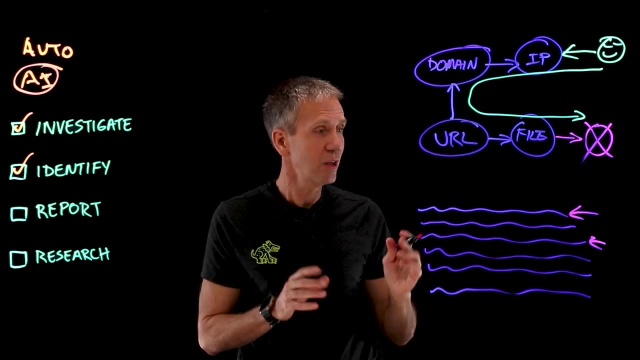 Well, in particular, what we'll find is in this case, let's go with an example and say: here is a record where a privileged user logged into the system and created a new account, Then almost immediately afterward, all the contents of a database, and then almost directly immediately they deleted the account. 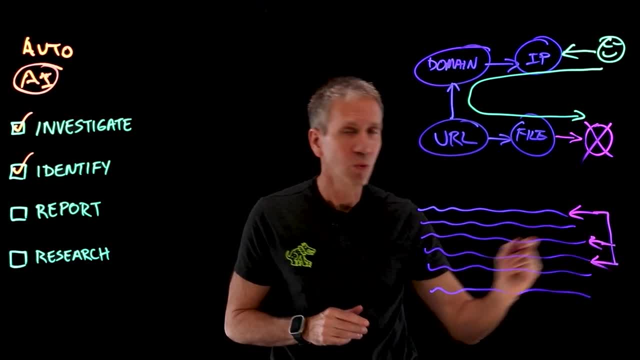 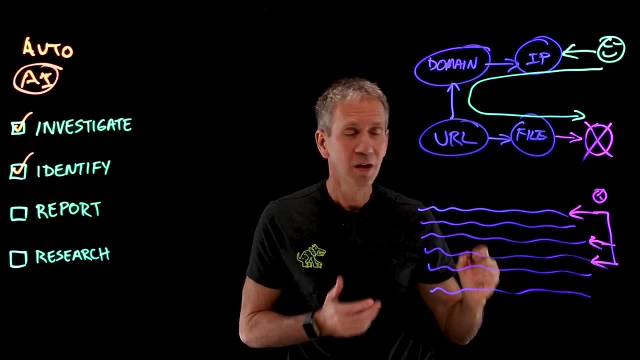 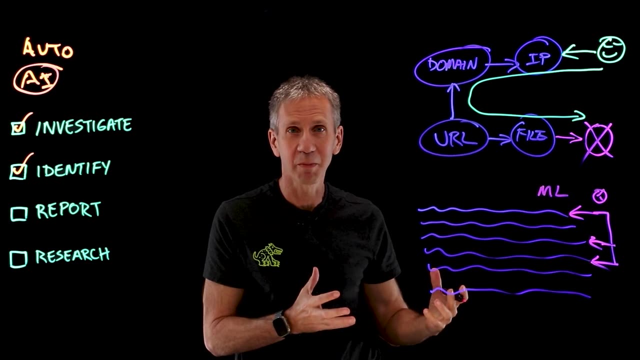 Now, each one of these activities independently wouldn't represent necessarily a problem, But if you do all of these within a very short period of time, then we could use a time decay function and something like machine learning, which is essentially pattern matching on steroids, to look at all of these things. 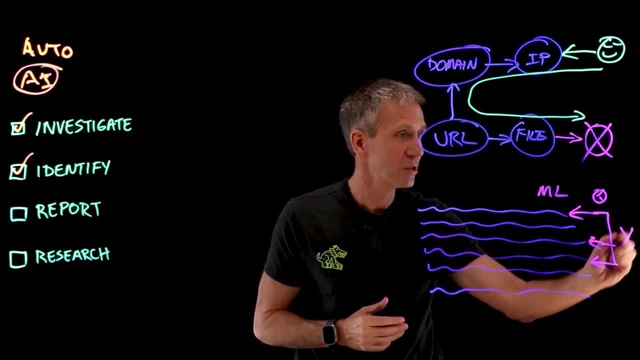 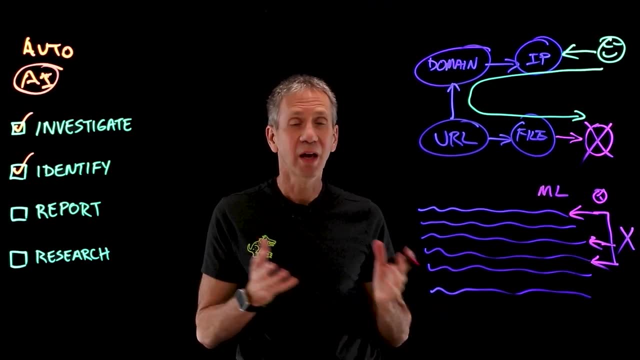 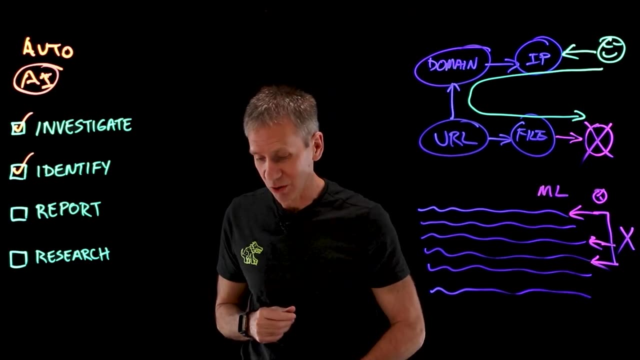 across multiple factors, across multiple records, and realize we have an outlier, We have an anomaly, We have what may be an attack scenario where an insider has taken advantage of the system. So that's another use of AI, and machine learning in particular, in order to diagnose a problem. 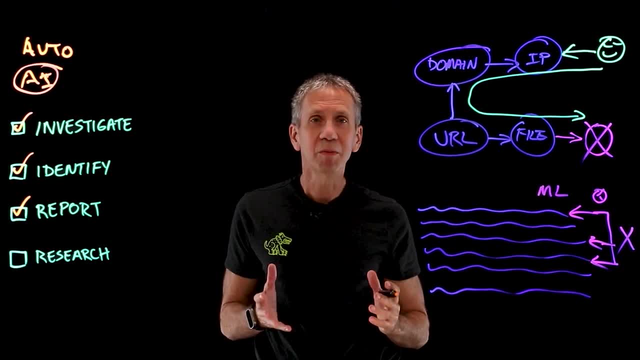 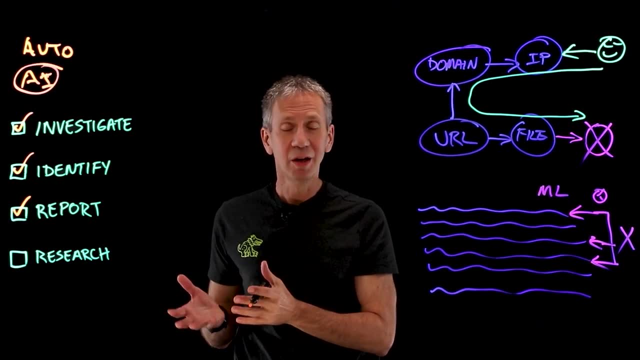 What else could we do? Well, we could report. There's a requirement in security circles that you report against- Are you complying with regulatory requirements or not- And some of the things that we might do in those cases is rather the log records and process those. 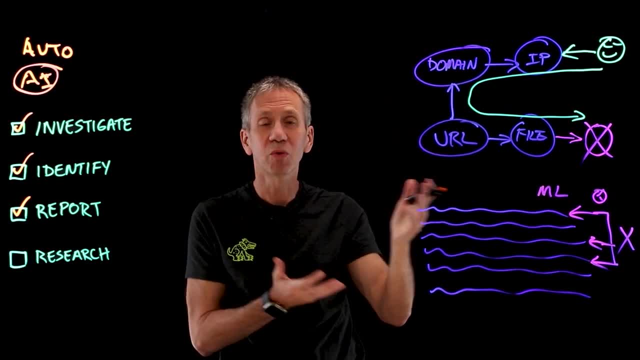 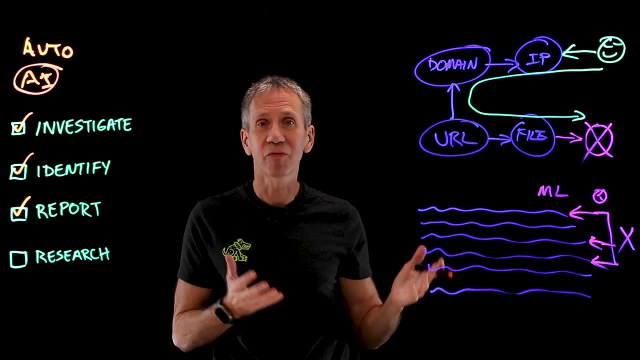 We might also use information that we've gained here to enrich our reporting data. So that's another example: We're enriching the reports with the information we have from the AI system, And that's also allowing us to report with spending less time. 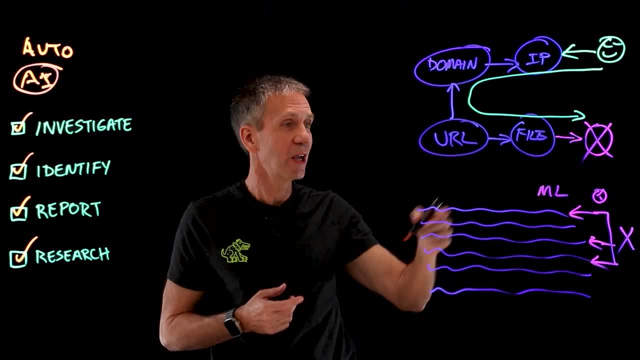 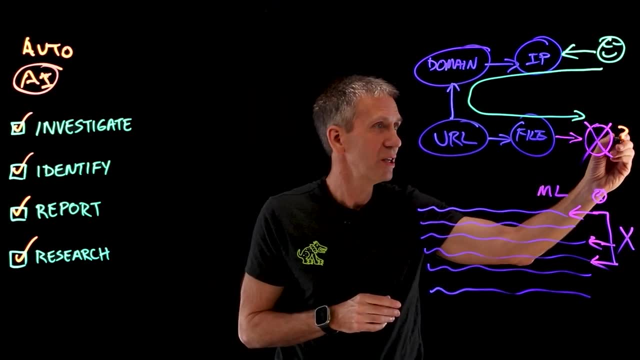 And then, finally, to do research. Imagine I'm investigating, I'm identifying, I'm doing all these kinds of things, And what I'd like to be able to do is find out what, what is this bit of malware, And I'd like to know more about it. 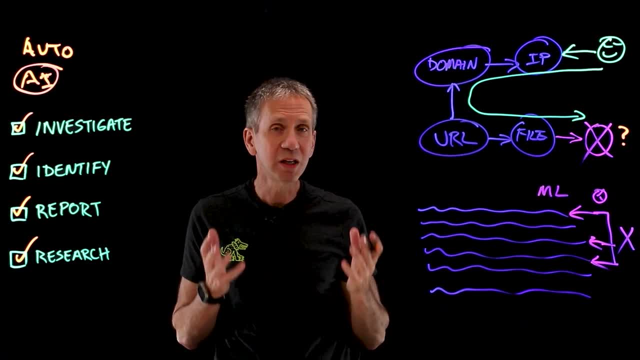 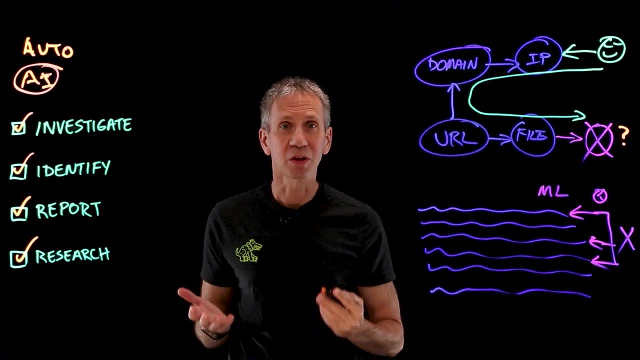 I want to know more about any of these systems, So it would be nice if I had a natural language processing system, a chat bot, that I could go and talk to and ask it questions, And it has a knowledge base that it draws on.